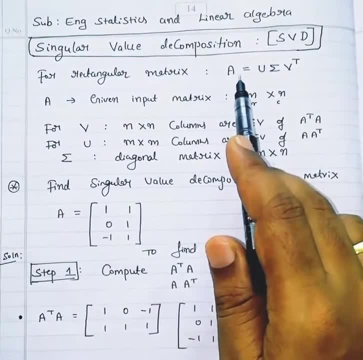 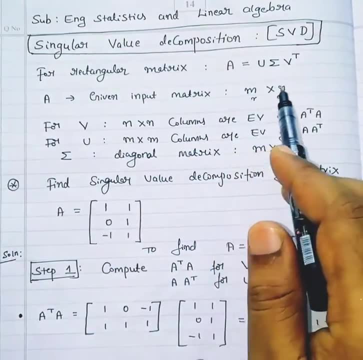 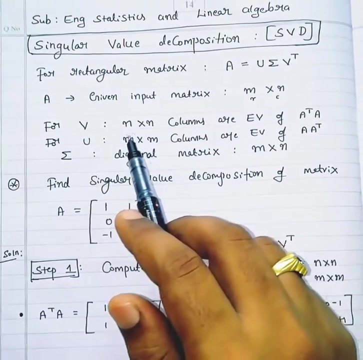 method is applied for rectangular matrix where the formula is a is equal to U summation, and VT where a is a given input. matrix of order. what m cross n? m is number of rows, n is number of columns for V. n cross n for U. m cross m for V, we. 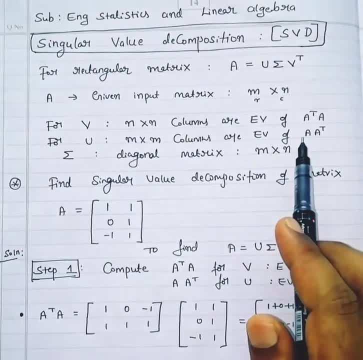 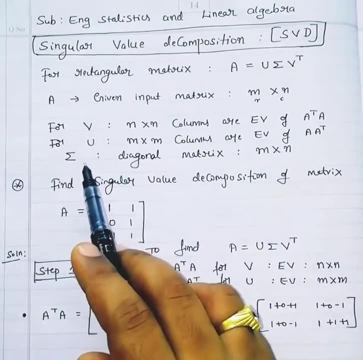 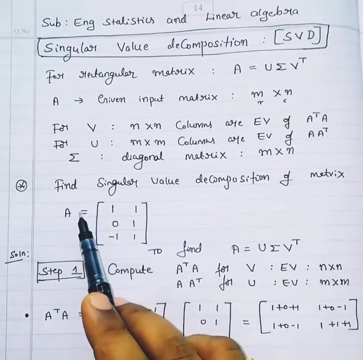 are calculating a transpose into a for U. we are calculating a into a transpose summation. diagonal matrix m cross n. where this symbol is diagonal matrix is having m cross n order. so we have to take on the problem. find the singular value, decomposition of matrix a. so what? 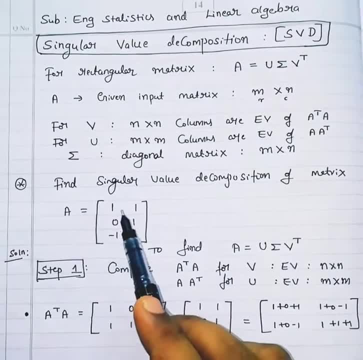 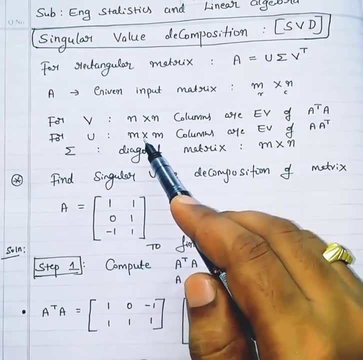 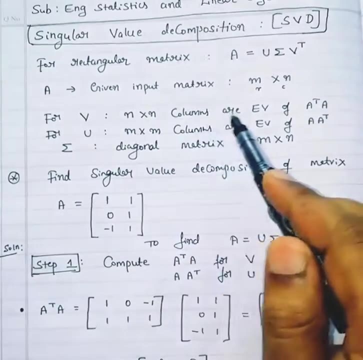 is the exact meaning of singular value. decomposition is: they will give one matrix. you have to decompose this matrix a into three parts. one matrix is U, which is m cross m, another is diagonal matrix, which is m cross n, and other is V, T, which is n cross n. so we will split this given matrix into three sub matrix. we 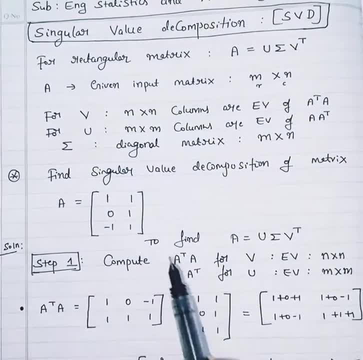 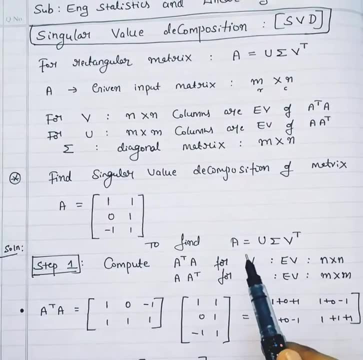 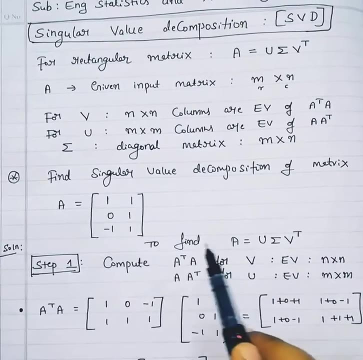 will see that. how to do that. what is step number one? as I told, we have to compute 80 into a. and it is for what? matrix? V matrix. look at this RHS. we have to calculate VT, so before that I have to calculate V. for this V we have to form, we have to find 80 into a. so 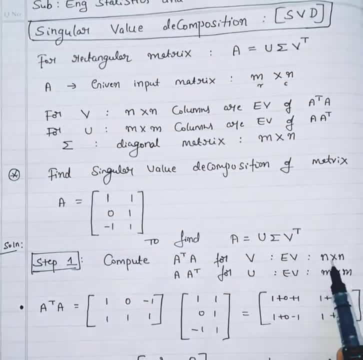 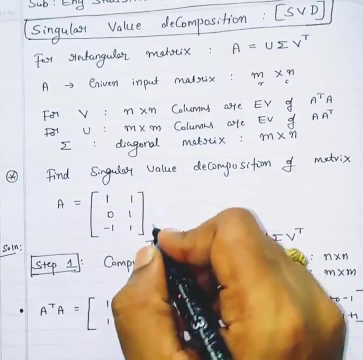 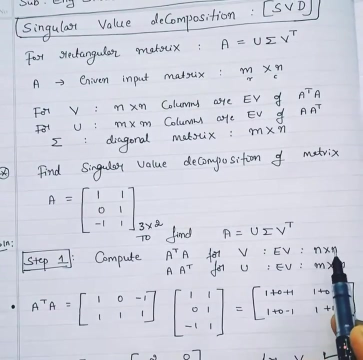 which is a eigen vector, and n cross, and we will see what is this eigen vector and n cross n n cross, n stands for a 80 into a. you can cut here n cross n. what is the given matrix? given matrix is of rose 3 & column 2, correct next for this. 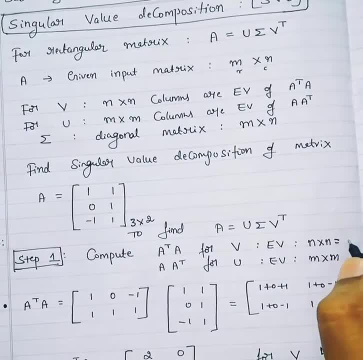 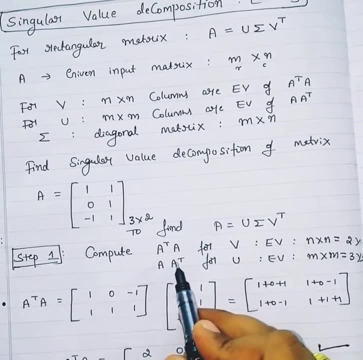 matrix. what is 80 in today? what is n cross n becomes n cross n becomes two cross two and this becomes three cross three. so we have to calculate a into 80. for what matrix? you? where is you? you is here and it is m cross n, 3 cross 3. so 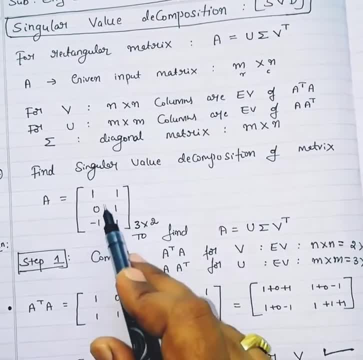 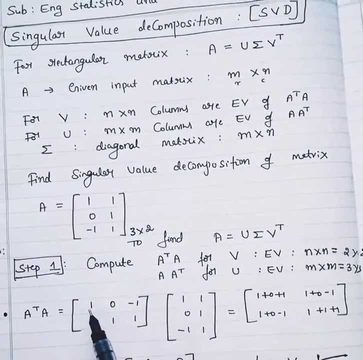 first we will calculate 80 into a, eighty into a. take the air transmission, suppose interchange rows and columns and write it here, a as it is. multiplication, simple matrix, multiplication 1 into 1, 0 into 0, minus 1 into minus 1. i think you know this. you have to do this. 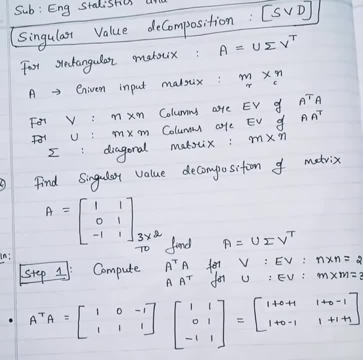 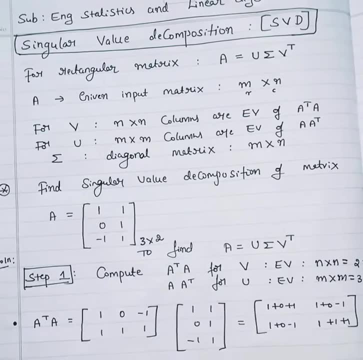 so what? the end result i got is 2 0, 0, 3. so here rows and columns. how many it is? 2 rows and 2 columns. look at here: it is n cross n. that is what exactly i have written here: n cross n, which is 2. 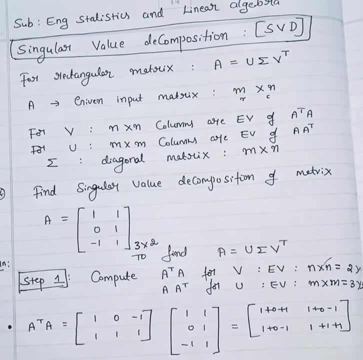 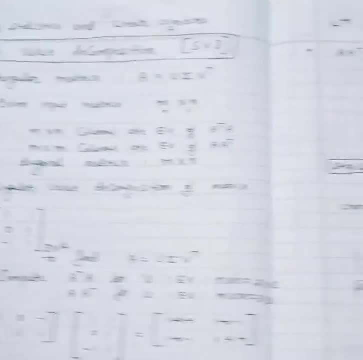 cross 2 and for which matrix? the matrix is going to be v here, so it is for 80 into a 2. cross 2 we will get and it is v. similarly, we will calculate it for a into 80. now, so a make it transpose, do. 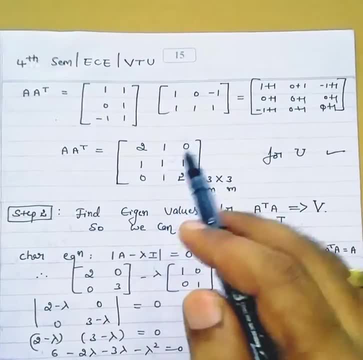 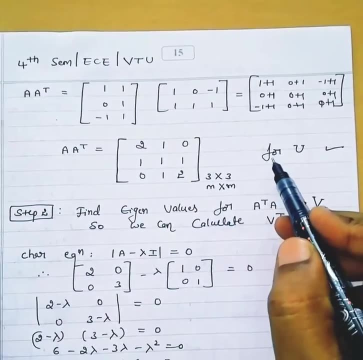 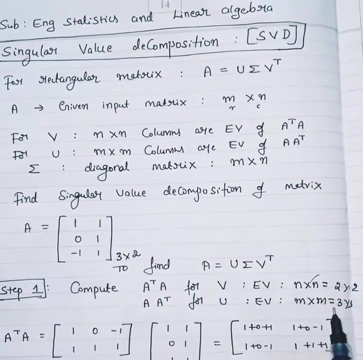 the matrix multiplication you will get. the resultant matrix is going to be like this, but number of rows and columns are 3 and 3, so it is 3 cross 3, m cross m. and for which matrix? for a u. so here you can just look at here for u, what is m cross m. so it is 3 cross 3 for a into 80. 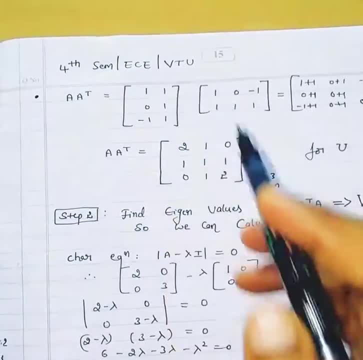 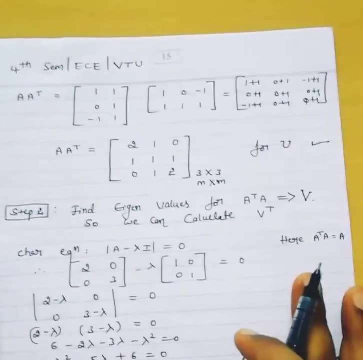 for a into 80, we got 3 cross 3. so this is what the step number one, step number one is exclusively. we have to compute 80 into a and a into 80. once we found, we have to find the step number to find the. 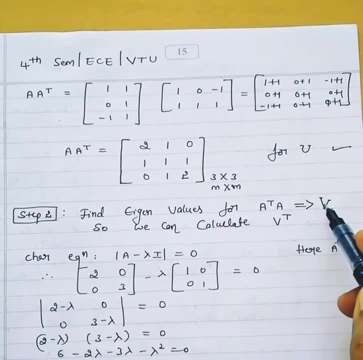 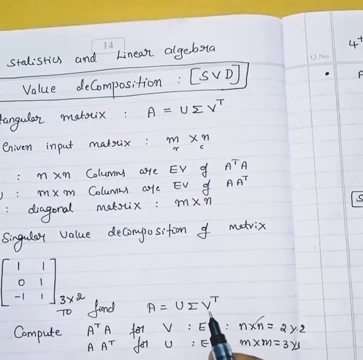 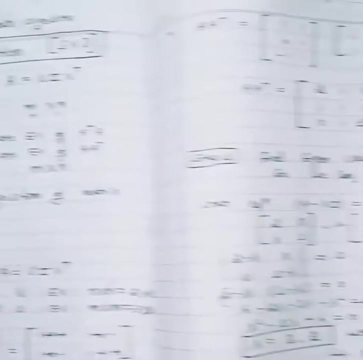 eigenvalues for 80 into a, which corresponds to which vector v, because we have to calculate what vt what is our final, ultimate aim is? we have to find this rhs. so here we have v and here we have to find v. transpose v corresponds to which matrix 80 into a. hence we have to find the eigenvectors of 80 into. 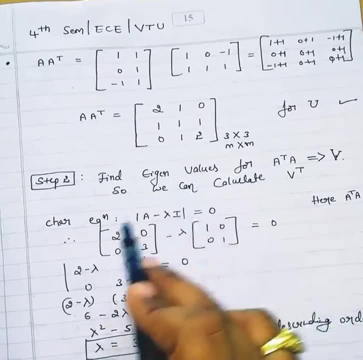 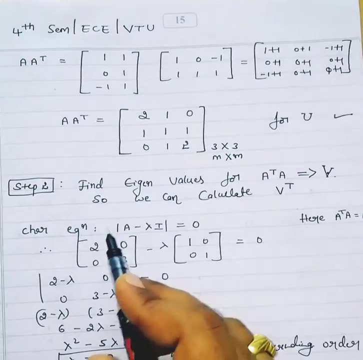 a. so here how to calculate the eigenvalues is: we will use the characteristic equation: determinant of a minus lambda is equal to 0. so here: 80 into a is a. so what is the 80 into a? 80 into a is which we got here. 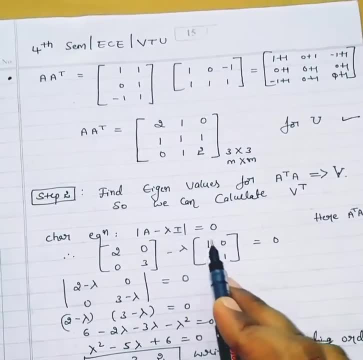 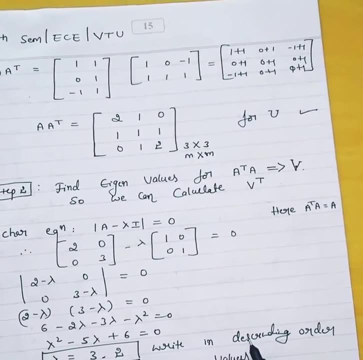 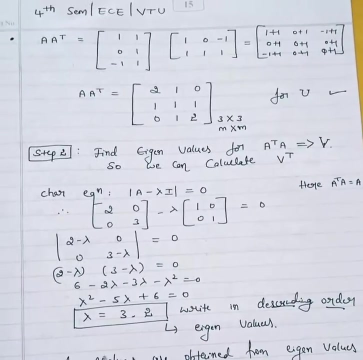 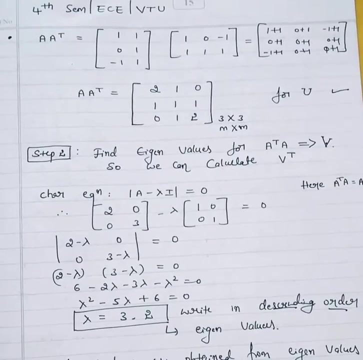 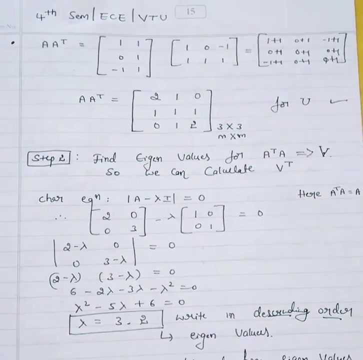 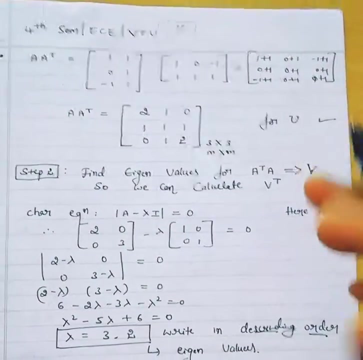 a is a L element of a minus A plus A, Y, c, rhs and 1 a p to our singular values. then obtain the eigenvectors for the eigenvalues, as like in the previous problems. once we calculate the eigenvalues, we are going to calculate the eigenvectors. so obtain the. 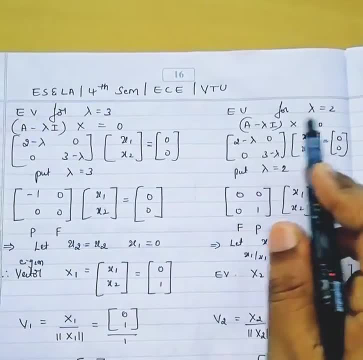 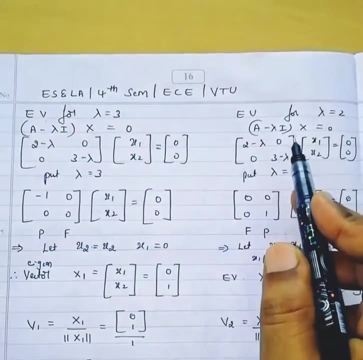 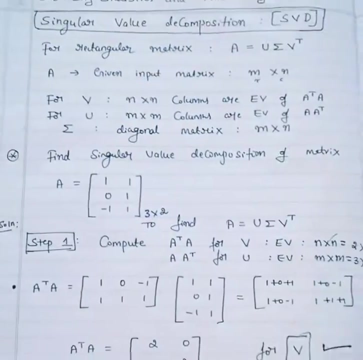 eigenvectors. so eigenvector for lambda 3, eigenvector for lambda is equal to 2. eigenvector: we have the formula a minus lambda i into x. x is a column matrix. so in the both the cases i have considered, just lambda is equal to 3. substitute here: what is a minus lambda i? a minus lambda i which we got here? 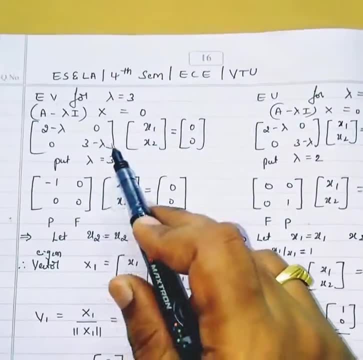 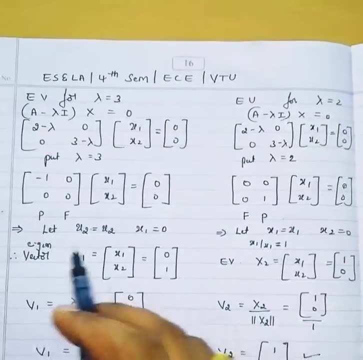 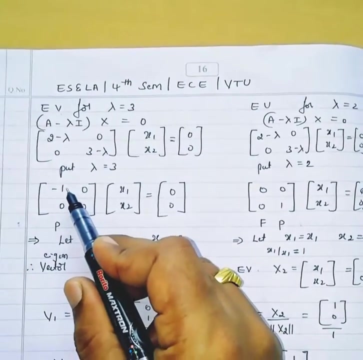 2 0 0, 3. so that is what, the same thing. just substitute lambda equal to 3, you will get this here. lambda equal to 2, you will get this up to here. the same precision here. observe these two. now we will search for the pivoted columns. this is pivoted column one. 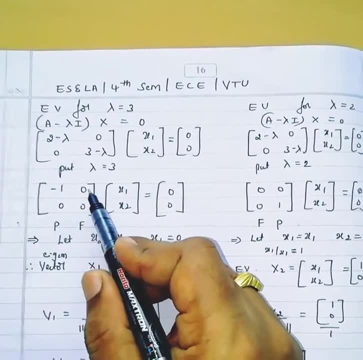 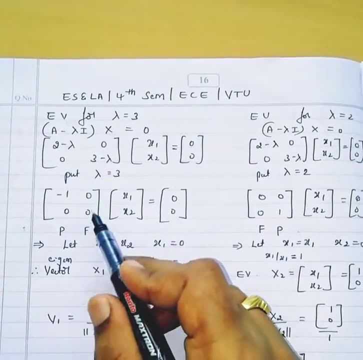 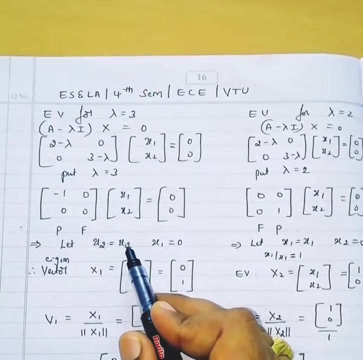 leading one. so here nothing is there. so it is free variable. so free variable. we will always: it is x2. it is x1 free variable. we will always assume. so let x2 is equal to x2. we will assume x1 as 0. when i take x2 divided by x2, what is the value 1? so x1 is 0 and 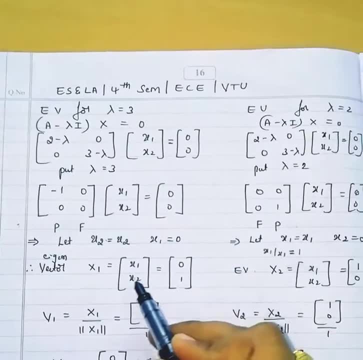 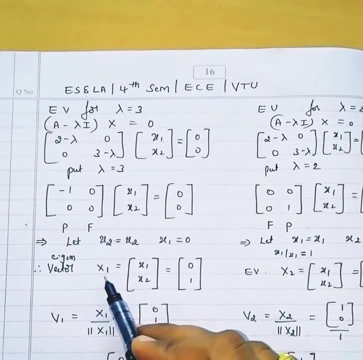 x2 is equal to 1. that's why eigenvector can be written as: x1 is equal to x1, x2. what is the value of x1: 0? what is the value of x2: 1? so this is what eigenvector we will got. get it for lambda equal to. 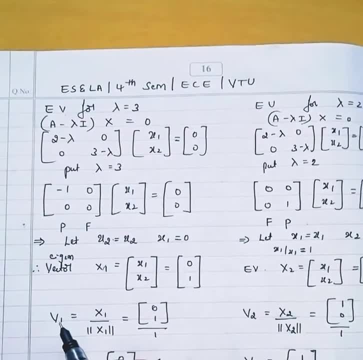 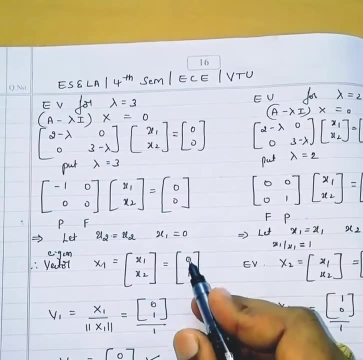 3. once we got the eigenvector x1, we will calculate v1. v1 is equal to x1 divided by magnitude of x1. x1 is as it is, magnitude of x1 is. it is square root of 0 square plus 1 square. so i will get it. 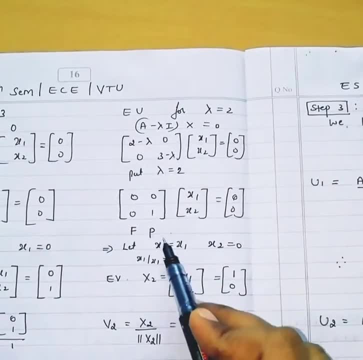 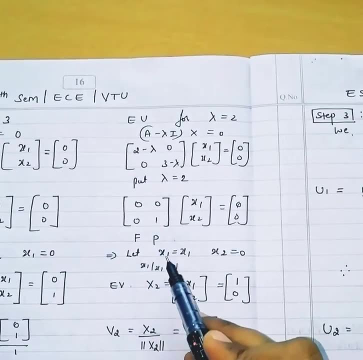 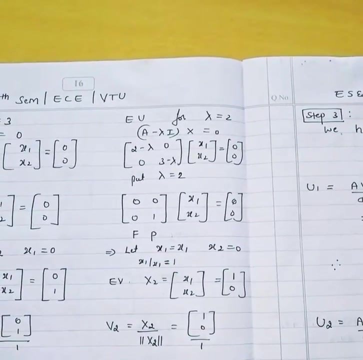 so v1 is equal to 0, 1. similarly here, just observe here: so here this is free variable because all entries are 0, so i will let: x1 is equal to x1 and this column i will take it as 0. so what is x1 by x1? it is going to be 1, so x2. eigenvector x2 is equal to x1, x2, so the x1 value. 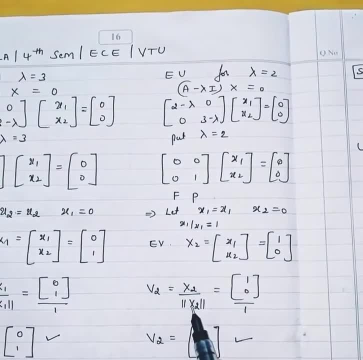 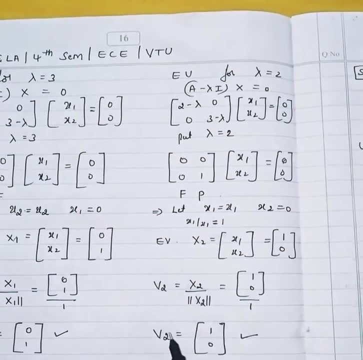 is 1 and x2 value is 0. so how to calculate v2- x2 by magnitude of x2? x2 is this: one. magnitude of x2 is calculated by root of 1 square plus 0 square is equal to 1, so v2 you will get. so once you get. 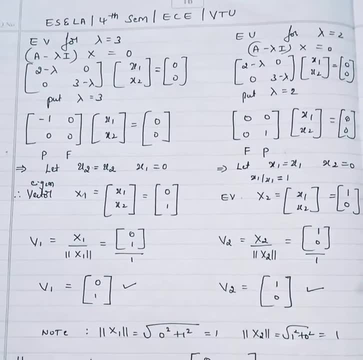 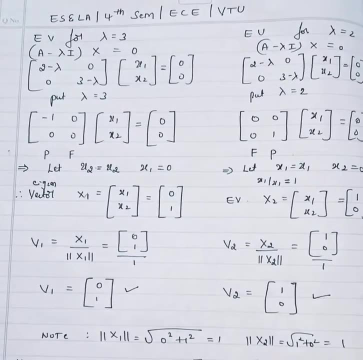 the v1 and v2. now we are going to consider the matrix. v is equal to, so right. for v1, what is the column eigenvector? you got 0 and 1. for v2, what is the eigenvector? you got 1 and 0. so overall, the 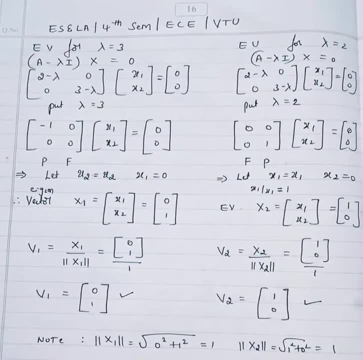 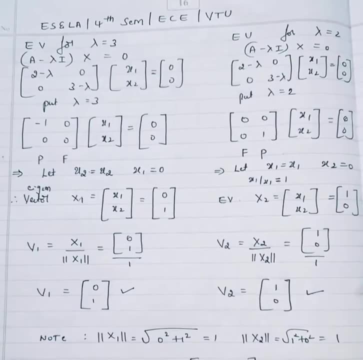 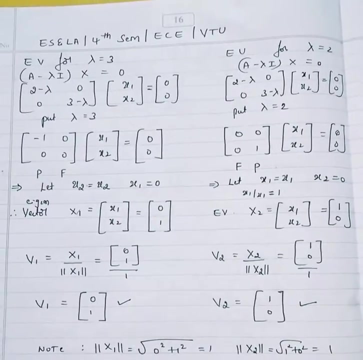 matrix we got is 2 cross 2, which is 0, 1 and 1: 0. why it is 2 cross 2. now i have written the note here. note for matrix v: n cross n, that is in this case n, means 2 cross 2. the columns are eigenvectors. 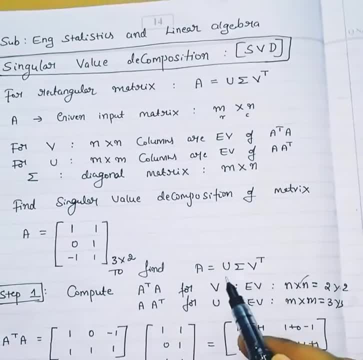 at into a. so we are speaking with respect to at into a. so we are speaking with respect to at into a, so we are speaking with respect to at into a. for v. the eigenvectors are what: n cross n means 2 cross 2 n means the number of. 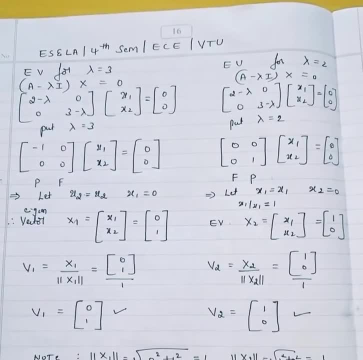 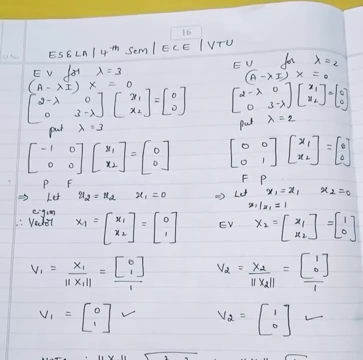 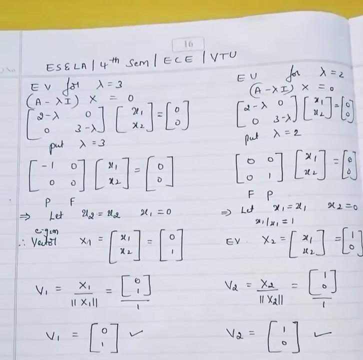 columns. so here, what is the number of columns? 2. that's what here n cross n. we are going to write for both rows and columns. it is going to be 2, but very important parameter in this case is columns. the columns are 2, so now what we are going to get is the transpose of v have to take. 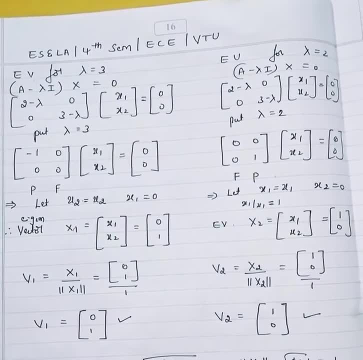 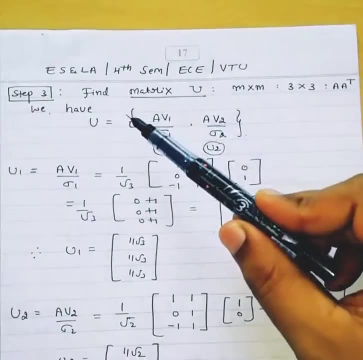 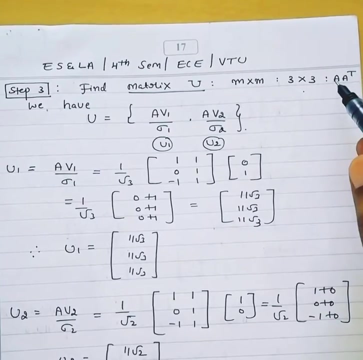 it. so v transpose is equal to 0, 1 and 1, 0. we will get. so first matrix, that is vt matrix we are going to get. next is step number 3. in the step number 3 we will find the matrix u? u is of order, what 3 cross 3? but we are calculating it for a. 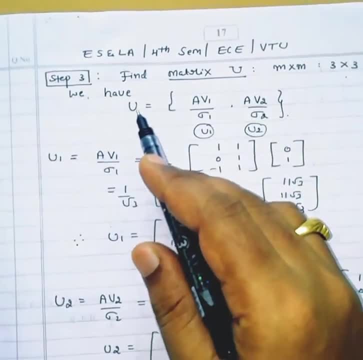 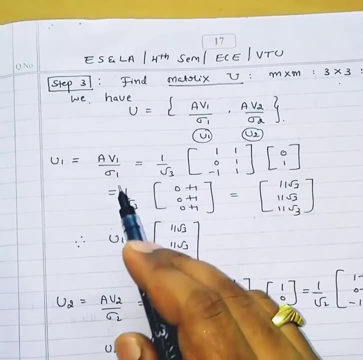 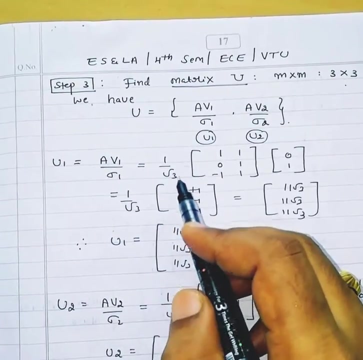 into a transpose. so here we are taking the u matrix first: u1 as a into v1 divided by sigma 1. u2 as a into v2 divided by sigma 2, so v1. i will calculate it separately. what is the value of sigma 1? we have calculated it singular value before root 1, by root 3 because of denominator. 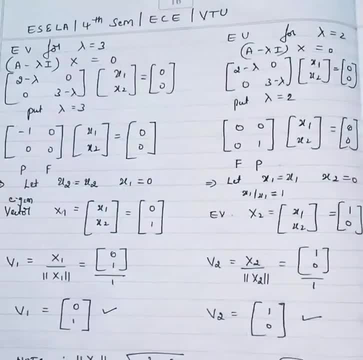 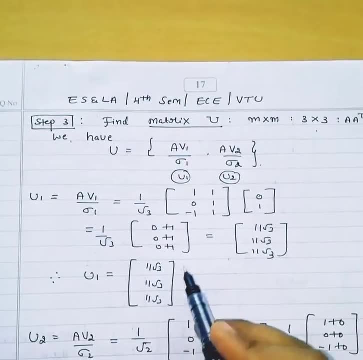 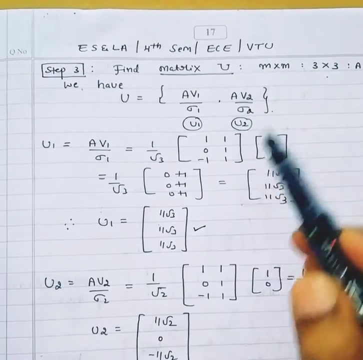 a value given matrix. v1 is which we have just substitute. we have calculated here v1, that will substitute here then after simplification. so here we are going to get u1 value as 1 by root 3, 1 by root 3, 1 by root 3. similarly calculate it for u2 a into v2 divided by sigma 2. so here sigma 2 is. 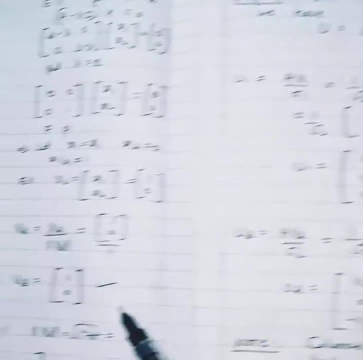 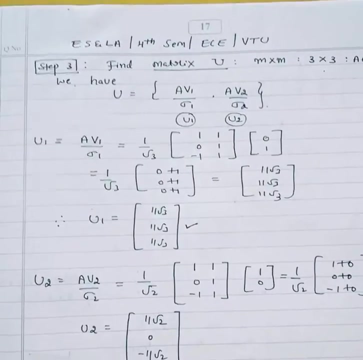 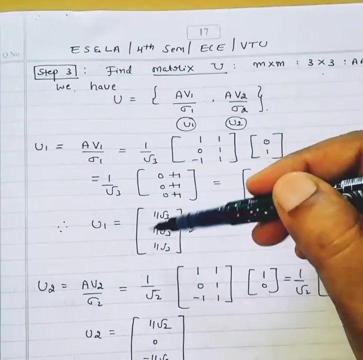 singular value. second, that is 1 by root, 2. similar process: v2, v2, v quote from this one. so we will 1, 0. so after calculation we will get u2 here. but very important thing, what we have to note here the columns of u are 3, cross, 3, matrix, but here the columns are only 2, that is. 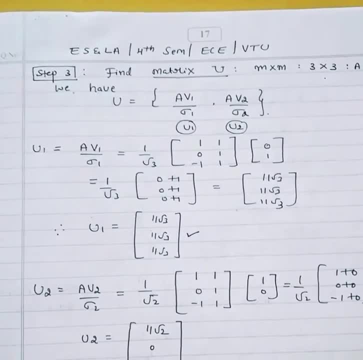 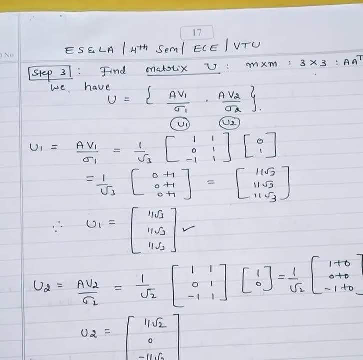 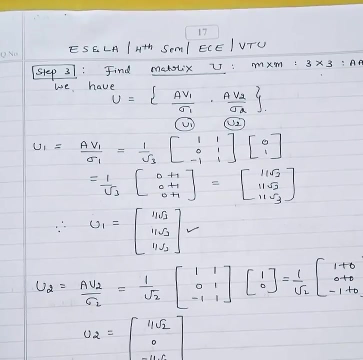 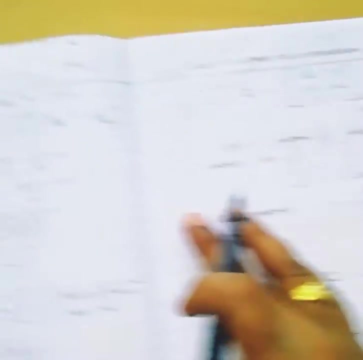 u1 and u2. where is u3? nothing, so it is absent here. so what we have to do is we have to take, we have to assume the v3 and we have to find the value of v3. so here, u3 is orthogonal to u1 and u2, so let u3. we have to assume initially alpha, beta and gamma, so once. 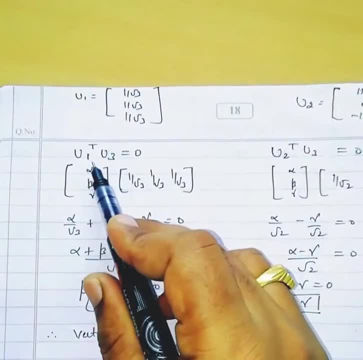 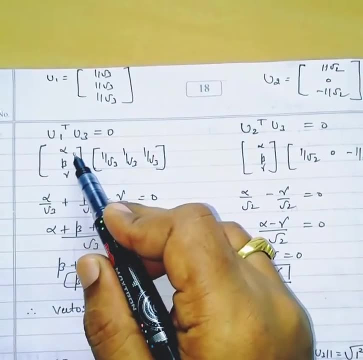 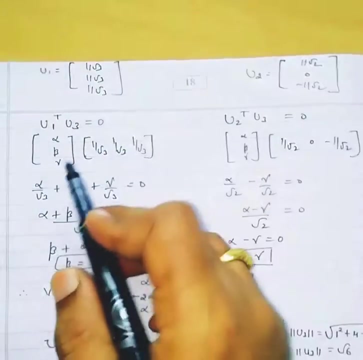 we have assumed, as we know, here the orthogonality between u1 transpose and u3 is 0 and u2 transpose, u3 is 0. so we are going to take that transpose alpha beta gamma as it is, transpose of u1 and here also same transpose of u2, so you can just have the matrix. 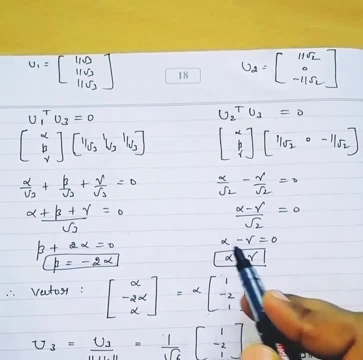 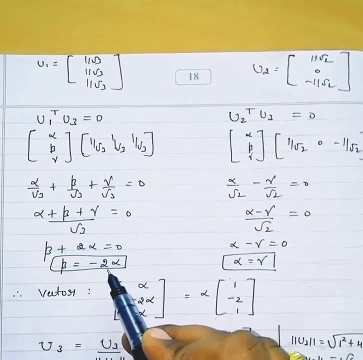 multiplication. you will get here like this. so from this what we will get is alpha minus gamma is equal to 0, so alpha equal to gamma. so if we substitute this format over here, so we will get: beta value is equal to minus 2 alpha, so the vector at the end, what you can write alpha is alpha. 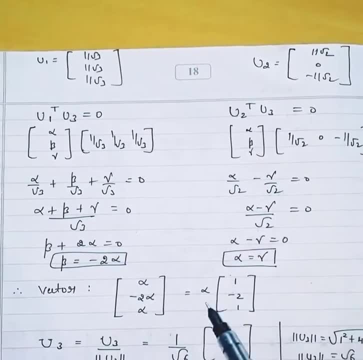 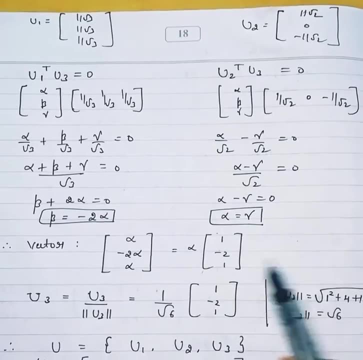 beta is minus 2, alpha gamma is alpha, so take out alpha common, so we will get 1 minus 2, 1. so at the end you will write what u3 is equal to u3. divided by magnitude of u3, what is the value of u3? same. 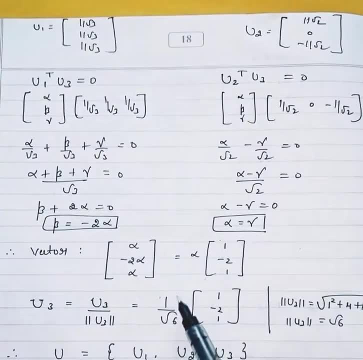 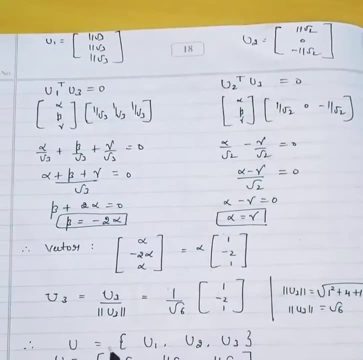 thing: 1 minus 2, 1. what is the value of magnitude of u3? it is equal to be 1 divided by root 6. so that is what 1 square 2 square plus 1. so it is root 3, root 6. so overall u matrix can be written as u1, u2, u3, so u is equal. 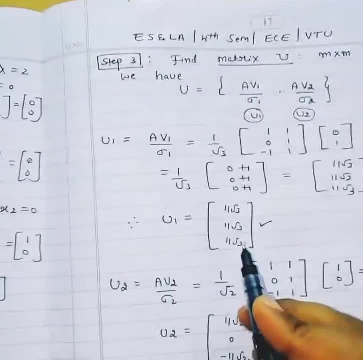 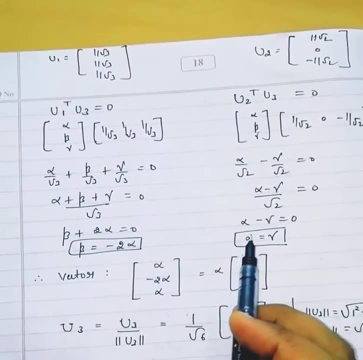 to u1. what is the value of u1, which you got here, this one, write it. what is the value of u2, which you got here? write it. what is the value of u3? we have assumed alpha, beta, gamma and those values we got here. so at the end, u1, u2, u3, we are going to write the matrix which is of 3 cross. 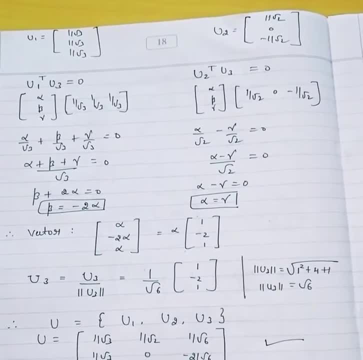 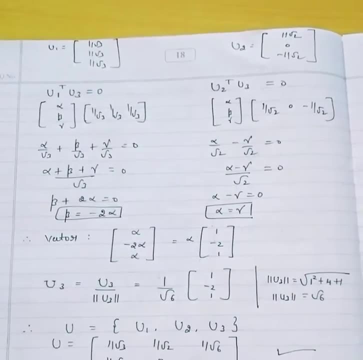 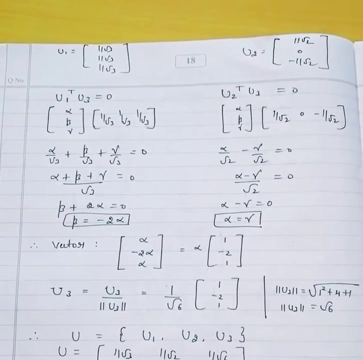 3. step 4 is to get the diagonal matrix summation, which is m cross n. so here we will write the singular values in the diagonal matrix, which which shows the diagonal elements. so in this case we got only two eigenvalues. hence 2, got only the two singular values. but what is the order of the? 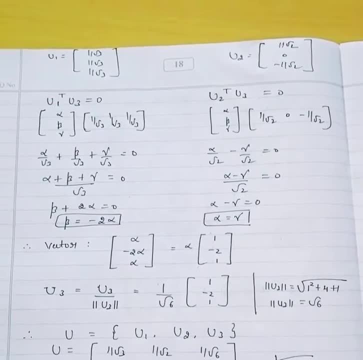 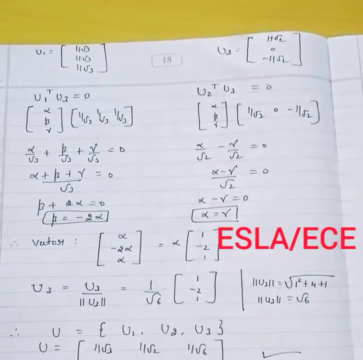 matrix: m cross n. in this case, what is m 3? what is n 2? so it is 3 cross 2, but we are having only 2. so what we have to do, we have to add one extra row so that you can make it 3 cross 2 matrix. so at the end you will get the diagonal matrix like: 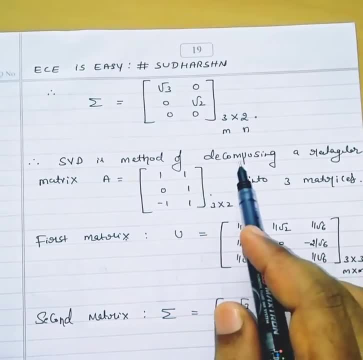 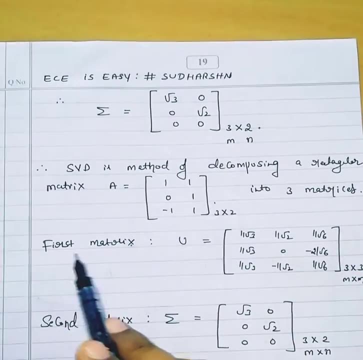 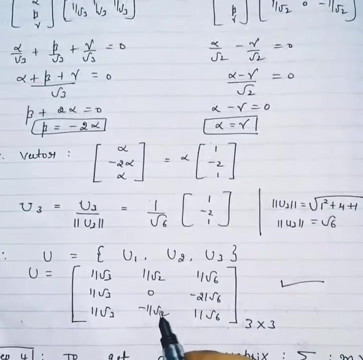 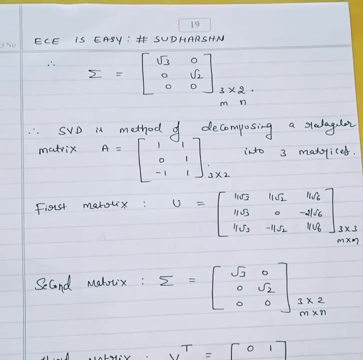 this therefore singular value. decomposition is a method of decomposing a rectangular, given matrix a, which is given, into three matrices. first matrix is: u is equal to, so what is what we got? the u matrix here. and the second is the second matrix, summation that has the diagonal matrix, which is 3 cross 2, and the third matrix transpose of v, which is 0, 1, 1, 0, 2 cross 2. 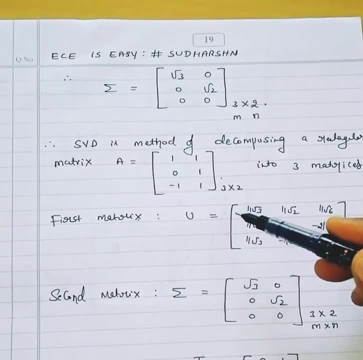 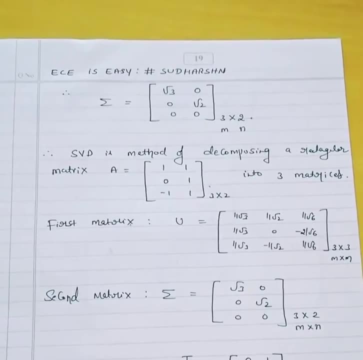 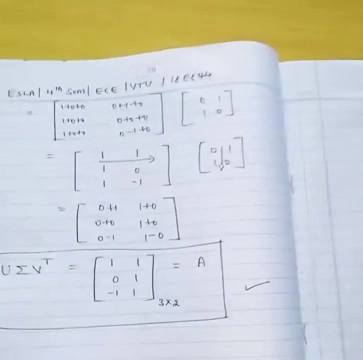 so if i decompose this matrix, we are going to get what? how many matrix? three matrix, first matrix, second matrix and third matrix. the last step is we can do the verification. for this. you can take this: u summation, vt substitute the value of v summation and vt go for the matrix multiplication.